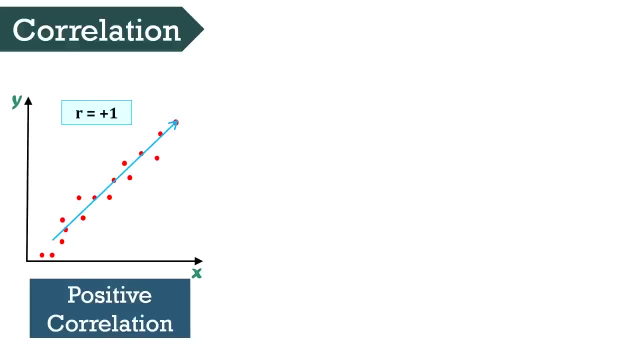 For example, height and weight, profit and investment, study time and marks obtained, yield and rainfall, electricity bill and temperature. Negative Correlation. Negative correlation represents the degree to which one variable increases when there is a decrease in another variable to form an inverse relationship. 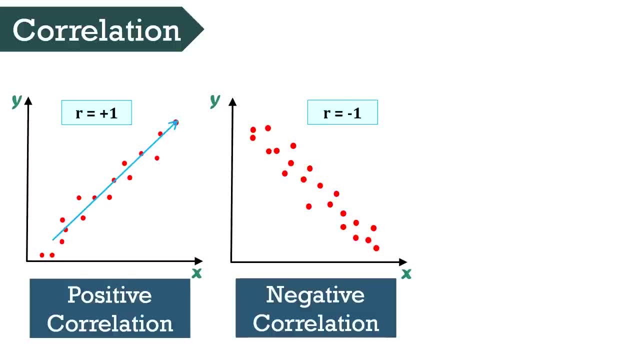 Hence in the case of inverse correlation. in the case of negative correlation, variables move in opposite direction, For example price and demand, speed and travel time, age and eye vision. Lastly, no correlation. Two variables are said to be uncorrelated when the change in one variable does not lead to any change in another variable in a certain direction. 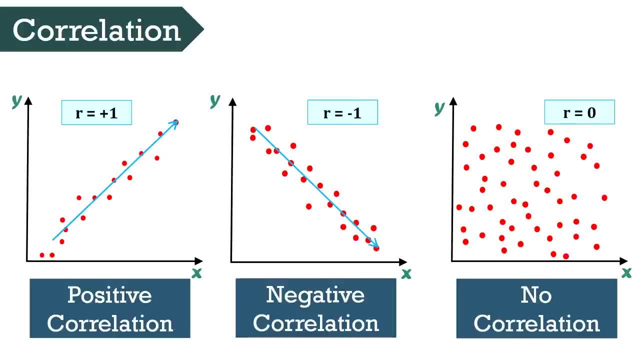 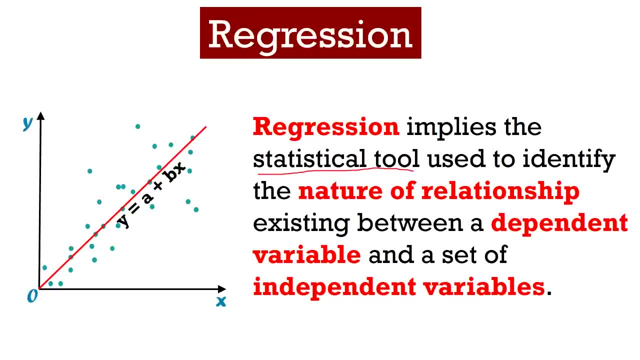 For example, age and intelligence, weight and energy, etc. Regression: Regression is a statistical tool used to identify the nature of relationship existing between a dependent variable and a set of independent variables. Here, dependent variable means the factor which the researcher attempts to understand or predict. 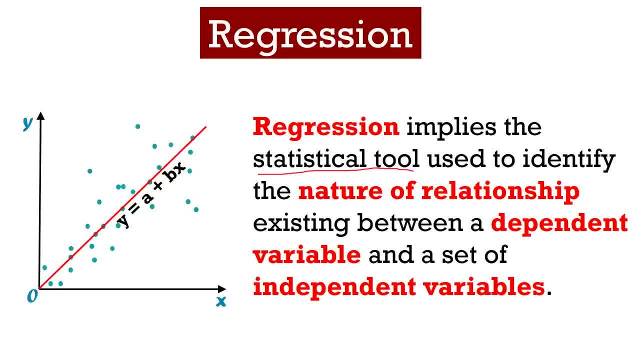 It is also called, as explained, variable. On the other hand, independent variable refers to the variable which the researcher assumes and have an impact on the dependent variable. It is also called as predictor variable. Furthermore, regression analysis is a set of processes which identifies the variable that influences the topic of interest. 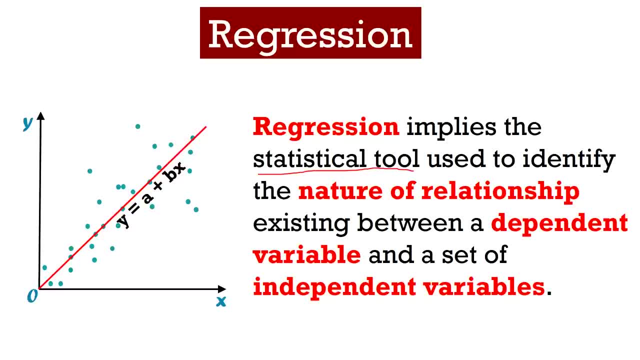 Hence one can ascertain which factors matter most, which are not to be considered, and how these factors influence each other. Regression Line: The regression line of y on x is the line of best fit for your data. That is, a line that represents the data points in the best way. 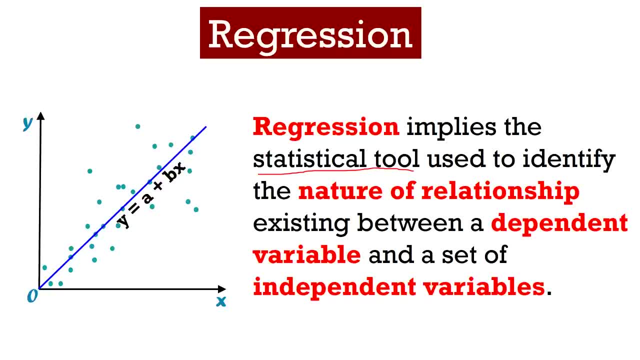 Derived by least squares method. it is used to predict the value of dependent variable y for the known value of independent variable x. In case of simple regression model, when y depend on x, then the regression line of y on x is represented by. y is equals to a plus bx. 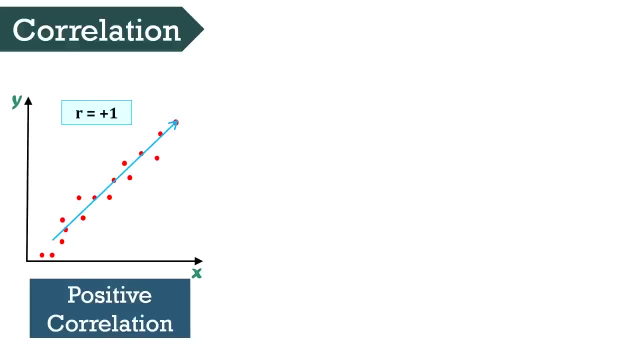 For example, height and weight, profit and investment, study time and marks obtained, yield and rainfall, electricity bill and temperature. Negative Correlation. Negative correlation represents the degree to which one variable increases when there is a decrease in another variable to form an inverse relationship. 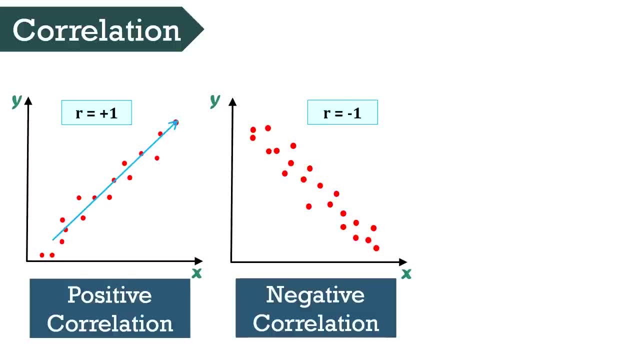 Hence in the case of inverse correlation. in the case of negative correlation, variables move in opposite direction, For example price and demand, speed and travel time, age and eye vision. Lastly, no correlation. Two variables are said to be uncorrelated when the change in one variable does not lead to any change in another variable in a certain direction. 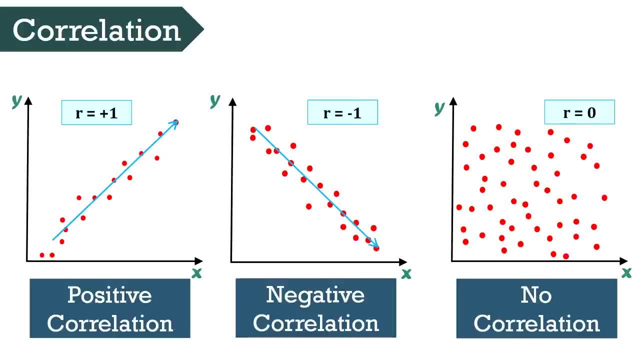 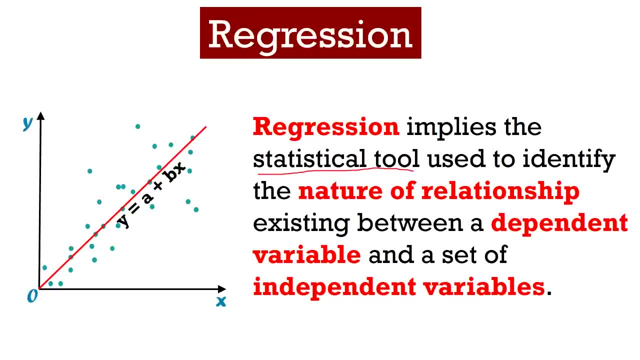 For example, age and intelligence, weight and energy, etc. Regression: Regression is a statistical tool used to identify the nature of relationship existing between a dependent variable and a set of independent variables. Here, dependent variable means the factor which the researcher attempts to understand or predict. 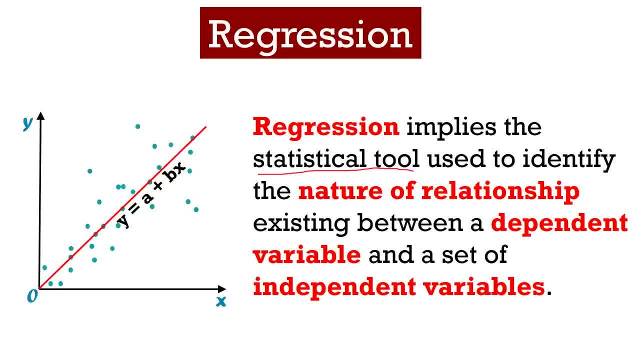 It is also called, as explained, variable. On the other hand, independent variable refers to the variable which the researcher assumes and have an impact on the dependent variable. It is also called as predictor variable. Furthermore, regression analysis is a set of processes which identifies the variable that influences the topic of interest. 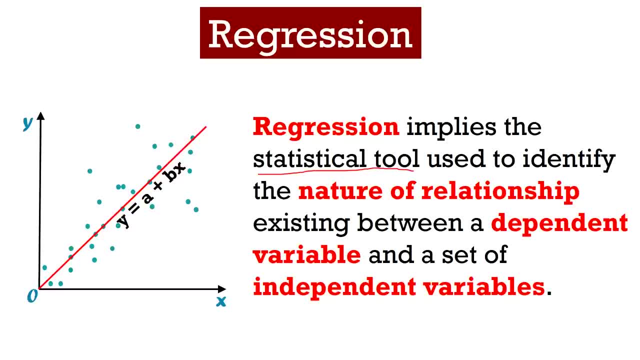 Hence one can ascertain which factors matter most, which are not to be considered, and how these factors influence each other. Regression Line: The regression line of y on x is the line of best fit for your data. That is, a line that represents the data points in the best way. 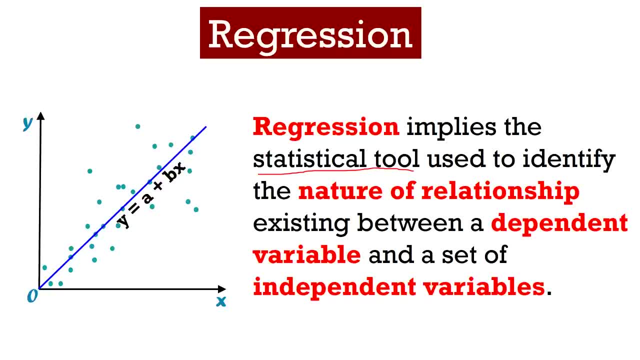 Derived by least squares method. it is used to predict the value of dependent variable y for the known value of independent variable x. In case of simple regression model, when y depend on x, then the regression line of y on x is represented by. y is equals to a plus bx. 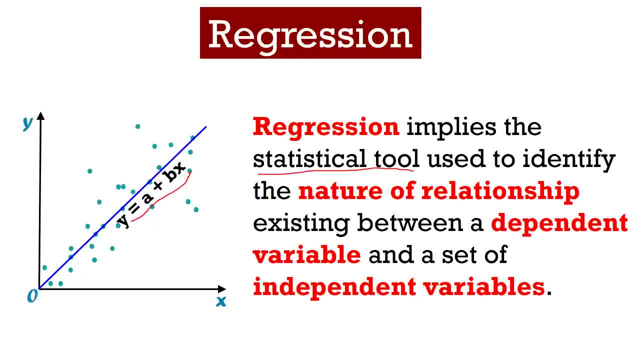 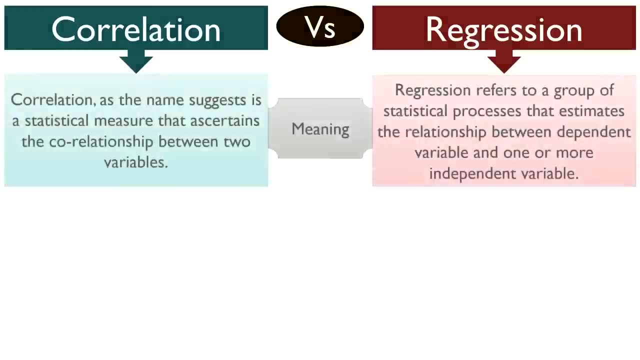 Where a and b are constants, commonly known as regression parameters. Moreover, b is also constant. Therefore, b is also called as regression coefficient of y on x. Now we are going to discuss the differences between correlation and regression. Correlation, as the name suggests, is a statistical measure that ascertains the correlationship between two variables. 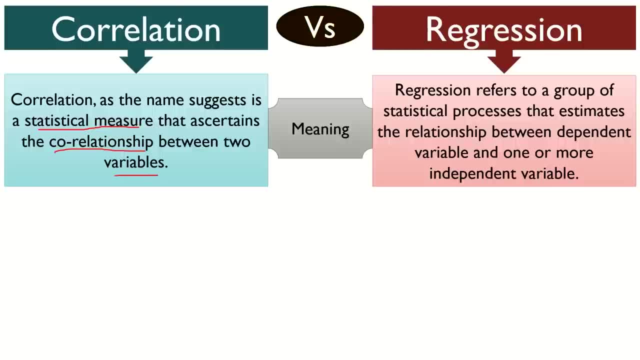 Correlation allows the experimenter to identify the association or absence of association between the variables under study. When two variables are found correlated, it helps in measuring the strength of association between the variables. On the other hand, regression refers to a group of statistical processes that estimates the relationship between dependent variable and one or more independent variable. 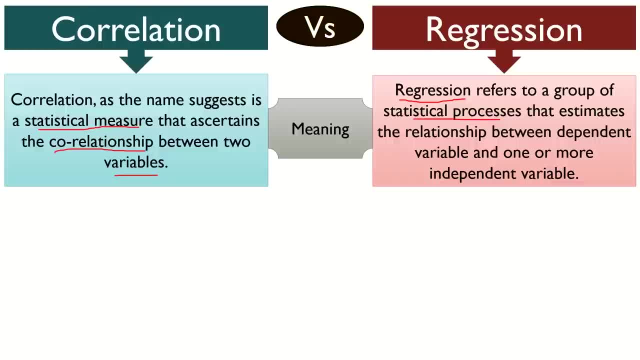 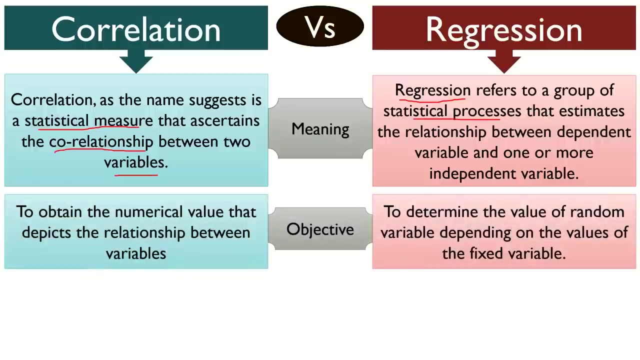 Basically, it represents how an independent variable x is numerically related to dependent variable y. Regression analysis helps to identify the functional relationship between the two variables So as to estimate the unknown variable with the help of known variable and make future projections. The main objective of correlation is to obtain the numerical value that depicts the relationship between variables. 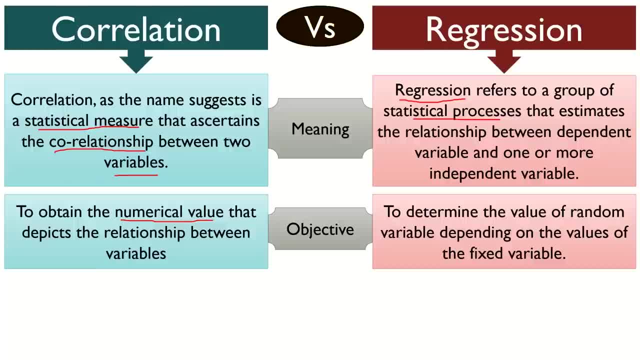 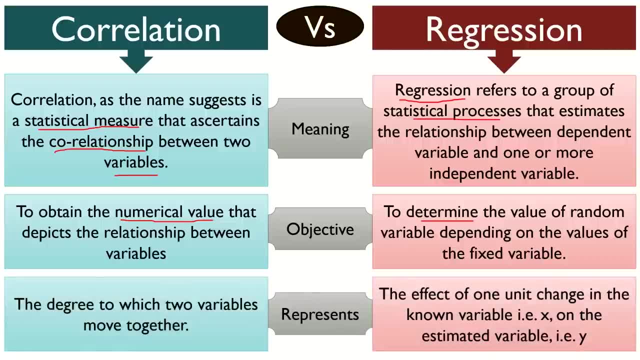 On the other hand, the main objective of regression analysis is to determine the value of random variable depending on the values of fixed variable. Correlation is a mathematical method. Correlation represents the degree to which two variables move together. as against, Regression represents the effect of one unit change in the known variable x on the estimated variable y. 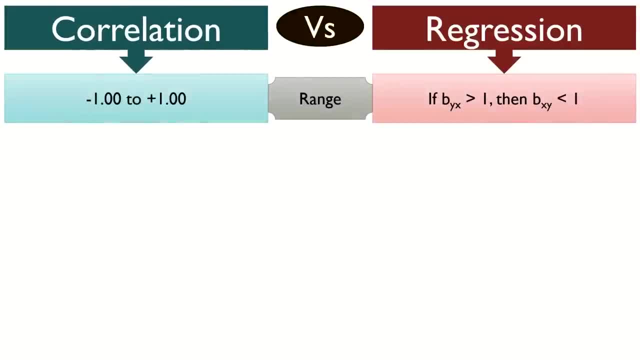 Next, correlation coefficient can range from minus one to plus one, Whereas if regression coefficient of y on x is greater than one, then regression coefficient of x on y is less than one. Coefficient Correlation coefficient is independent of any change of scale or shift in origin. 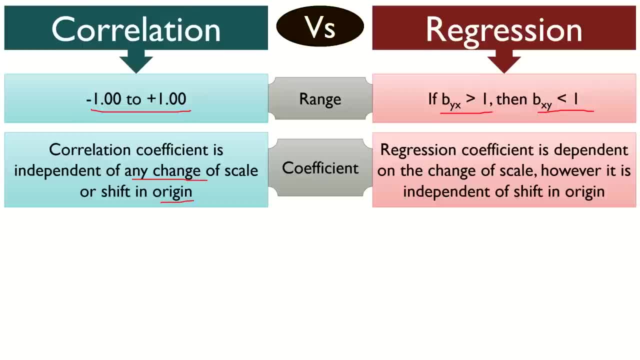 Conversely, regression coefficient is dependent on the change of scale. However, it is independent of shift in origin. When it comes to nature of coefficient correlation, coefficient is mutual and symmetrical. This means that correlation between x and y is same as y and x. 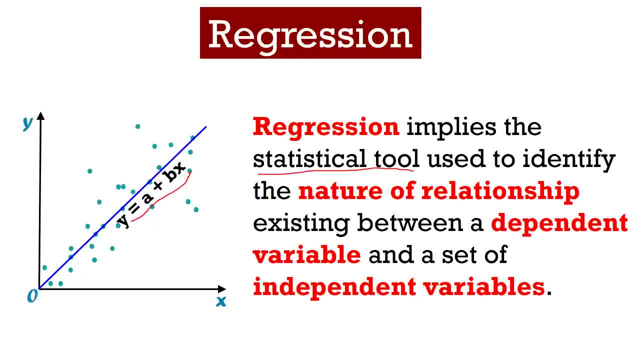 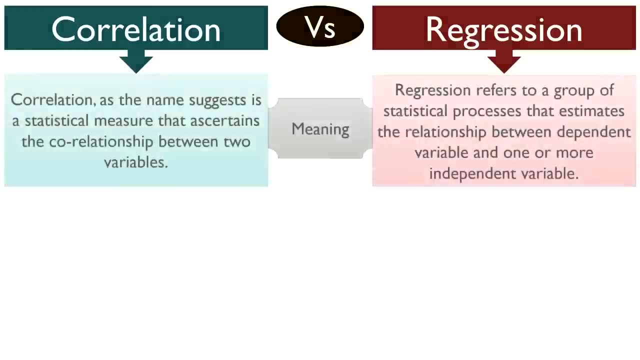 Where a and b are constants, commonly known as regression parameters. Moreover, b is also constant. Therefore, b is also called as regression coefficient of y on x. Now we are going to discuss the differences between correlation and regression. Correlation, as the name suggests, is a statistical measure that ascertains the correlationship between two variables. 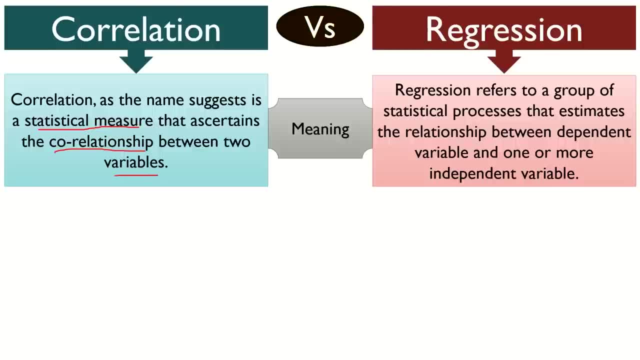 Correlation allows the experimenter to identify the association or absence of association between the variables under study. If the variables are found correlated, it helps in measuring the strength of association between the variables. On the other hand, regression refers to a group of statistical processes that estimates the relationship between dependent variable and one or more independent variable. 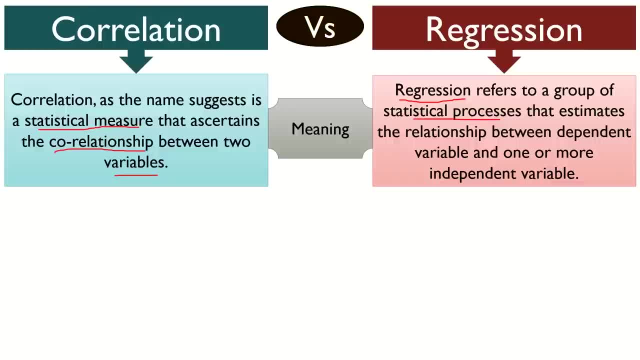 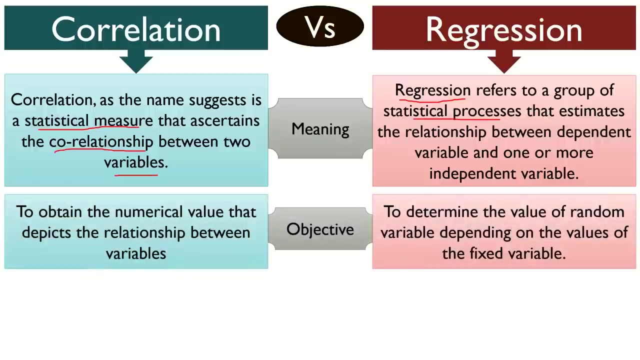 Basically, it represents how an independent variable x is numerically related to dependent variable y. Regression analysis helps to identify the functional relationship between the two variables So as to estimate the unknown variable with the help of known variable and make future projections. The main objective of correlation is to obtain the numerical value that depicts the relationship between variables. 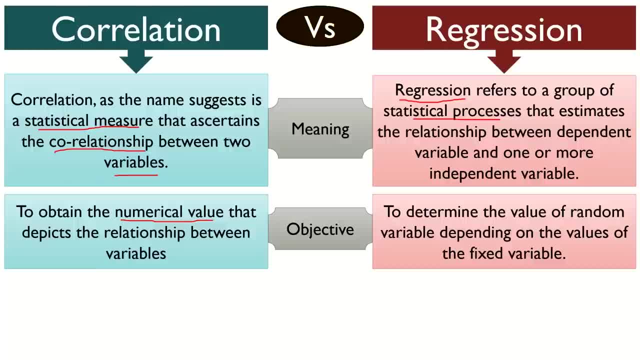 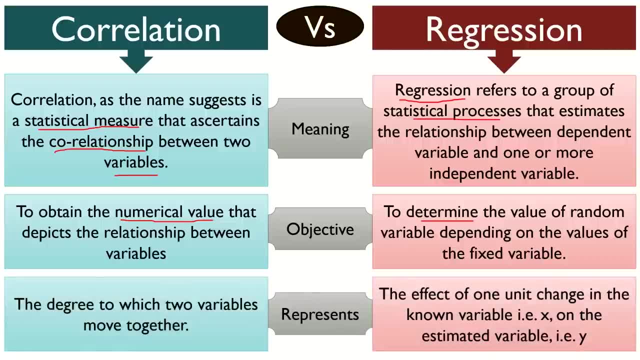 On the other hand, the main objective of regression analysis is to determine the value of random variable depending on the values of fixed variable. Correlation is a mathematical method. Correlation represents the degree to which two variables move together. as against, Regression represents the effect of one unit change in the known variable x on the estimated variable y. 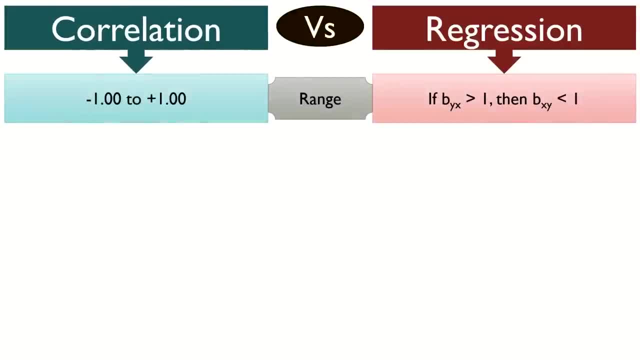 Next, correlation coefficient can range from minus 1 to plus 1.. Whereas if regression coefficient of y on x is greater than 1, then regression coefficient of x on y is less than 1.. Coefficient- Correlation coefficient- is independent of any change of scale or shift in origin. 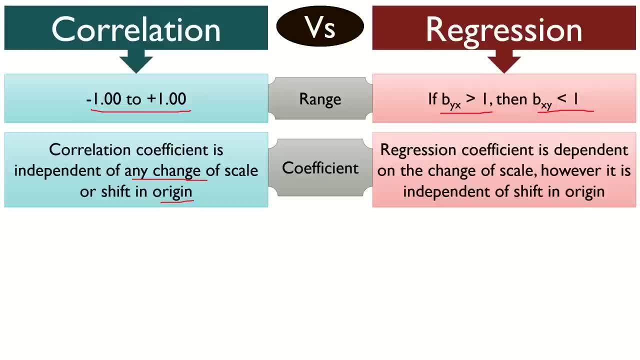 Conversely, regression coefficient is dependent on the change of scale. However, it is independent of shift in origin. When it comes to nature of coefficient correlation, coefficient is mutual and symmetrical. This means that correlation between x and y is same as y and x.